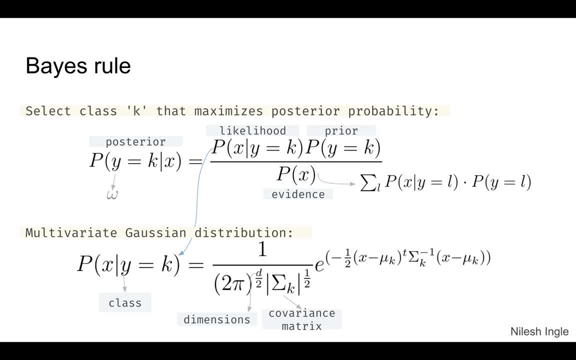 if the prior knowledge in that case would could be knowing that what type of vegetables were put into the hopper, so that we could use that in the model to update it so that the model is more accurate. another example could be if you are planning to go on a vacation and if we want to know the weather, so the prior knowledge in that. 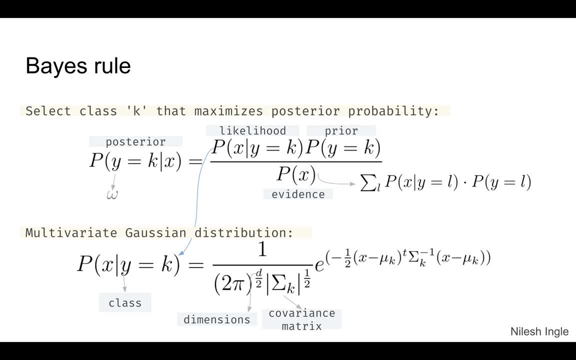 case could be. what was the weather like at that location last year? so that could be a prior knowledge. then we have the evidence, which is the normalizing term which is given here. what this does is it brings the values or this product in the numerator within a range of zero to one, and so the 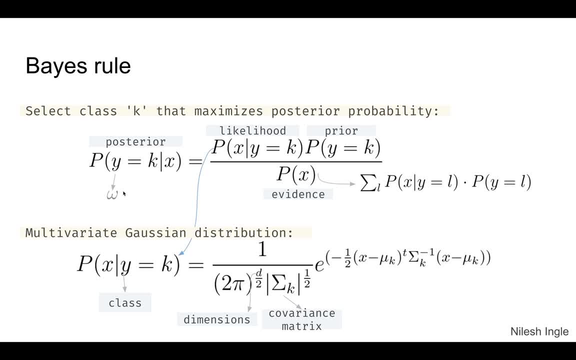 posterior probabilities would be in zero to one range. in the previous videos, We the Y was written as Omega, So this is notation from the cyclotron doc. So that's a change here and here we have all our capital piece In the previous video, very specific, and we have the View roku value. so you gotta see that. if you, for example, if we say you: 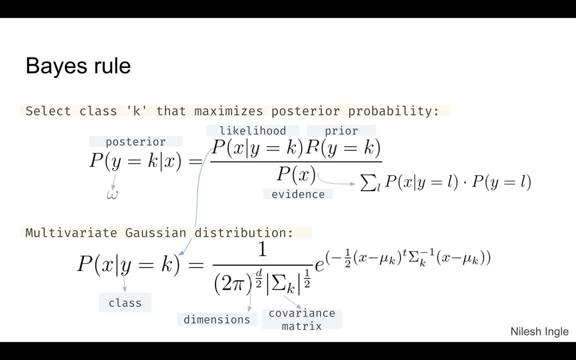 we had the probability mass function, so capital p, for the prior and posterior, and then for likelihood and the evidence term we had a small p, which is the probability density function. so here we'll go with what's in the docs for scikit-learn, and then below we have the equation: 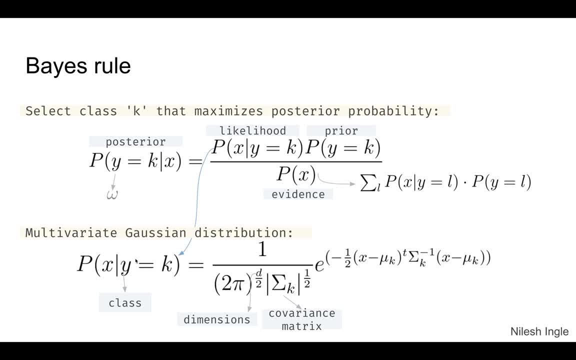 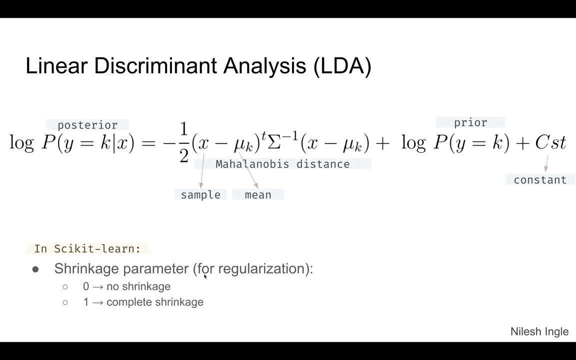 for multivariate gaussian distribution, and so here you can see that the sigma then is a covariance matrix, and again, these would be matrices right here. so for linear discriminant analysis, this was the equation that we discussed in the previous video, where what we are trying to maximize is the log posterior. 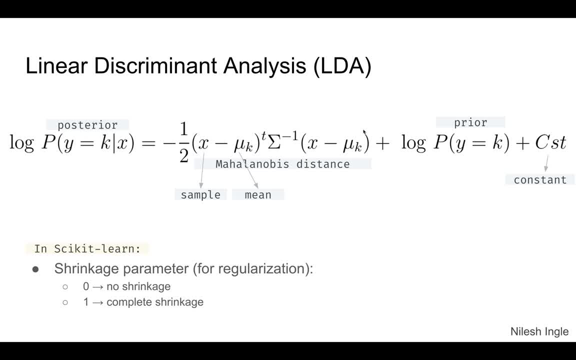 posterior probability, and that here we are using the mahalanobius distance, which is given by this term right here, and the special specialty of this distance is that it takes into account the variation in the data's data set. so that's why this covariance matrix is in here, and then we add that to the priors and then we have this additional. 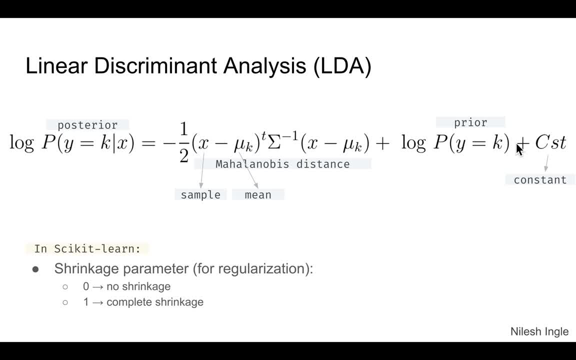 constant. that's written there now in the scikit-learn docs. we can use regularization parameters for this for when we implement this. so if we set it to zero, there's no regularization, so no shrinkage zero. and if it's set to one, then it's complete shrinkage. so that would start to underfit. 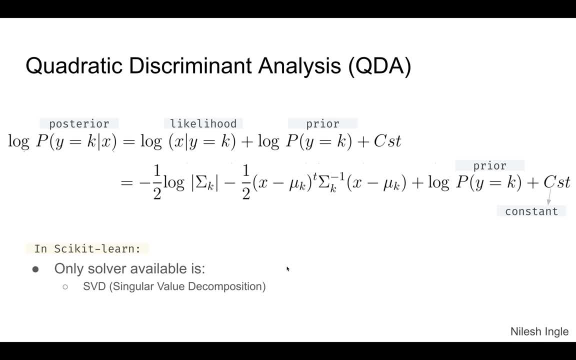 for quadratic discriminant analysis, again we have the equation for multivariate gaussian distribution and then below we have the given here and now, in this case, we have the log, we have the likelihood and the prior, and then these are: this is the final equation for that, and the difference is here we have this term. 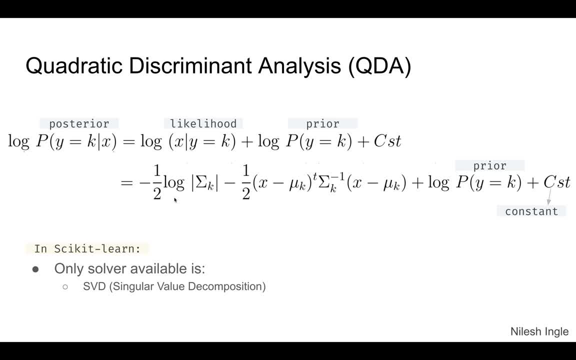 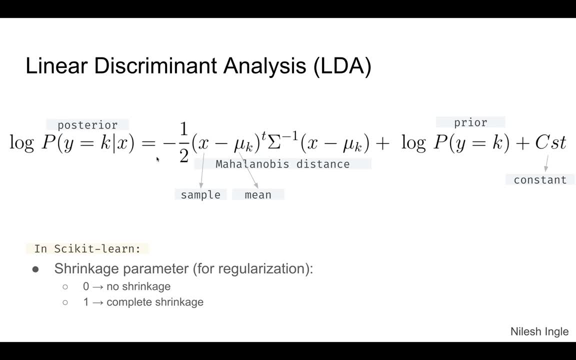 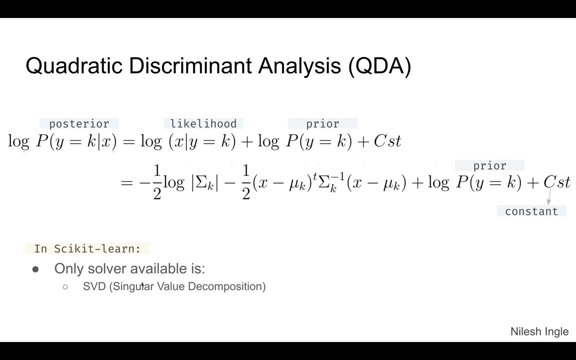 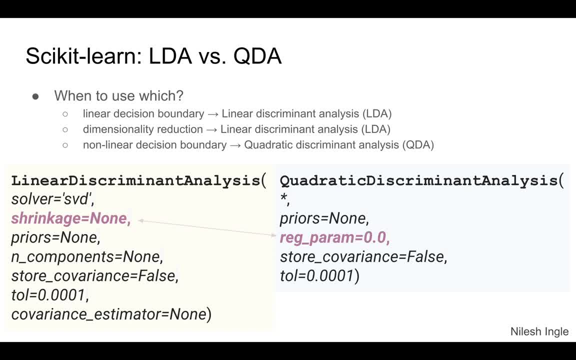 options. now, when do we use lda versus qda? so when? linear versus quadratic discriminant analysis? if your boundary, if your, if you need, if the data needs to be separated by a linear decision boundary, then lda would be a choice. if, however, the decision boundary cannot be linear, 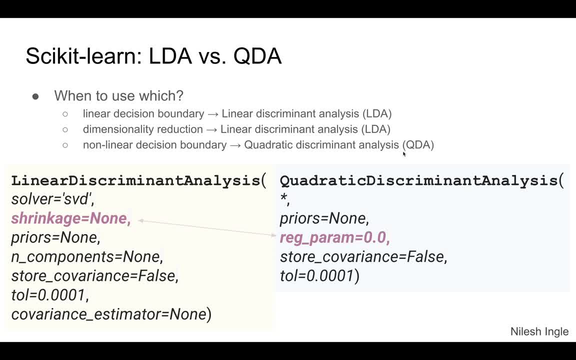 then quadratic discriminant analysis should work in those cases. additionally with linear discriminant analysis there is a function called attribute, called transform. that function called transform, that we can use with linear discriminant analysis to reduce the dimensionality, that is, to reduce the number of features in the data set, and then those reduced data set can then 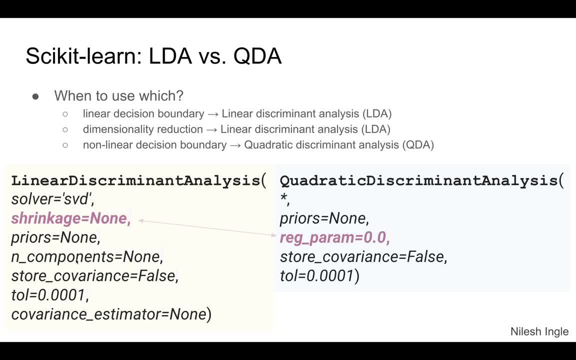 be used for training a model. and here is just the code for lda and qda where we can see that in qda the regularization can be done by setting values for the reg underscore param option, whereas in linear discriminant analysis there is a shrink shrinkage option that can be set. now for code. 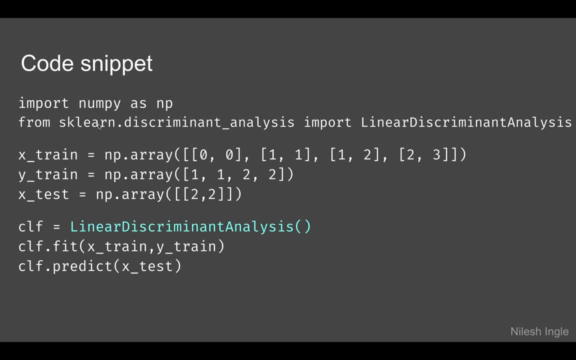 snippet at this time. so far, we have been importing linear underscore models. now that we are done with that and here we'll now for this video, we have a new library, so so sklearndiscriminant underscore analysis and we can import linear discriminant analysis as well. 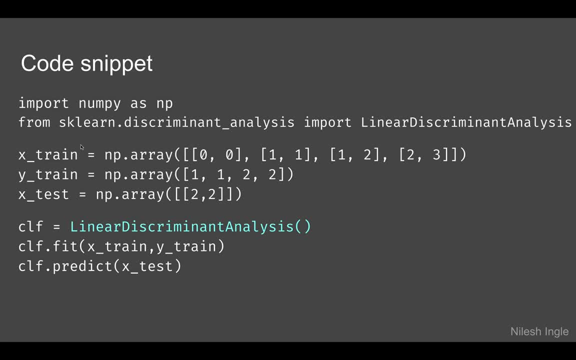 as quadratic discriminant analysis, and this stays the same. we have the x train, y train, train, x test and finally, we initialize the variable clf using this method and then fit it on x train, y train and then predict using the x test. now let's see how it works. 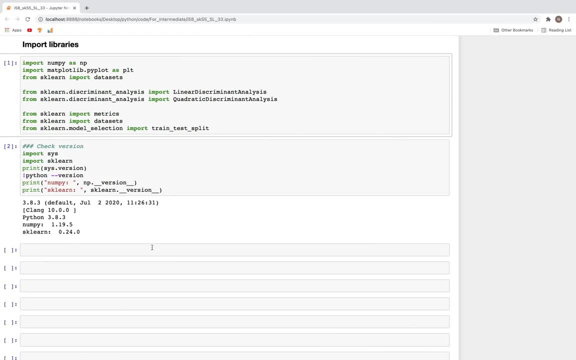 so let's get into jupyter notebook and see how we can implement these. i have imported a couple of libraries: numpy, matplotlib datasets and the new libraries are these two and additionally, these are working splitting the data and looking at the matrix. this got imported झ, and these are the versions that i'm using. 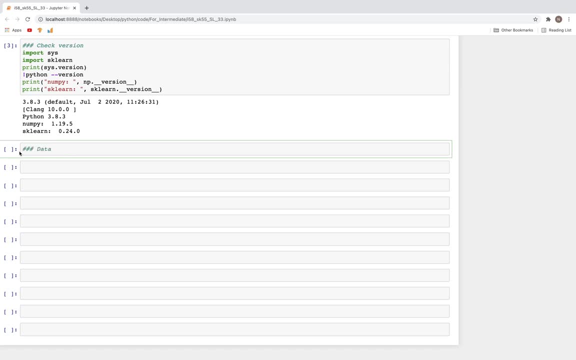 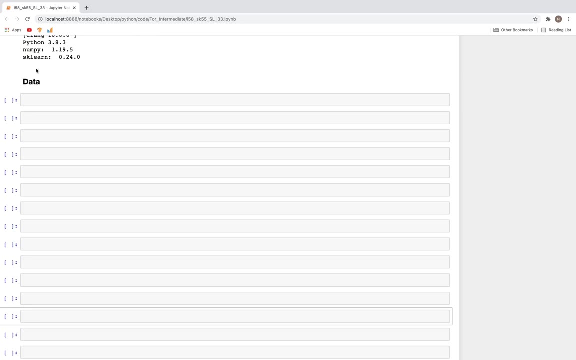 now for data. we'll keep it simple. uh. i'll use the i iris dataset so that we can focus on the uh how the method works. so for that let's import the get that uh data is equal to data sets. dot load underscore iris and uh. you probably already 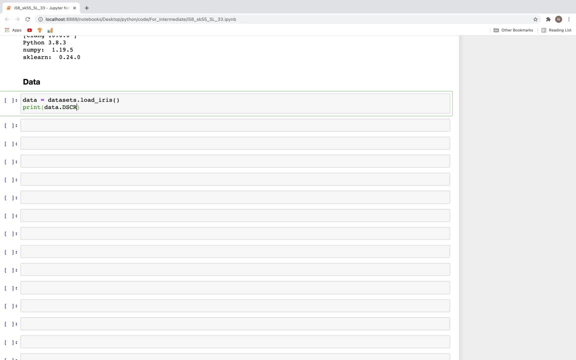 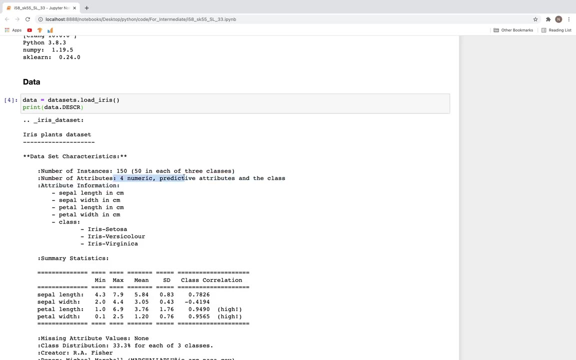 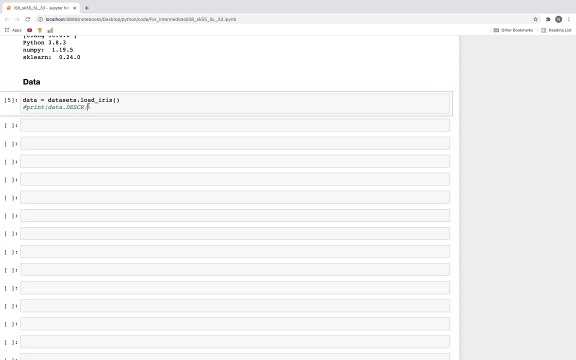 know this, so we can look at what the data is. so by typing d, e, s, c, r, and here we can see that there are, uh, four features, which are these, and then there is one class, which is this one- sorry, three classes, for this is the column for that, and with that we can split the data set. so x underscore. 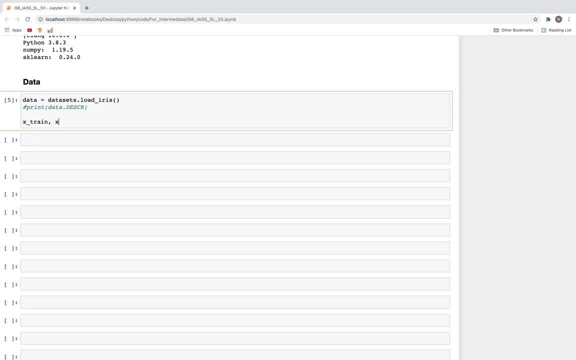 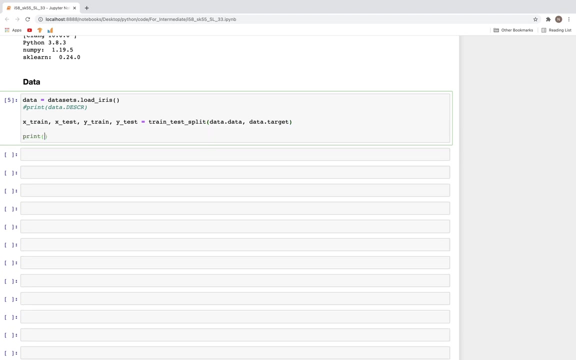 train x underscore test. y underscore train y underscore test is equal to train underscore test, underscore test, split data, dot data data dot target and this. with this we can also print the x train and y train shapes, because after we reduce the dimensionality, we'll notice that the shapes would be different. 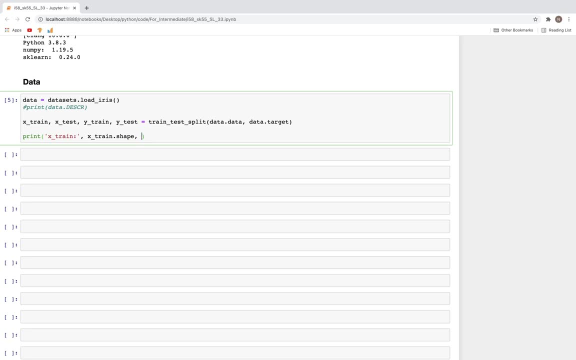 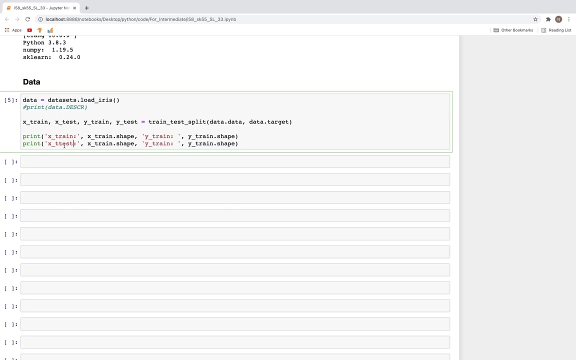 so x underscore train dot shape. and then we can also have the y underscore underscore train dot shape and y underscore train dot shape. and let me copy this so we can also get the shapes for the test data set. simply go ahead and replace this and type in test. so let me copy that and paste it here. 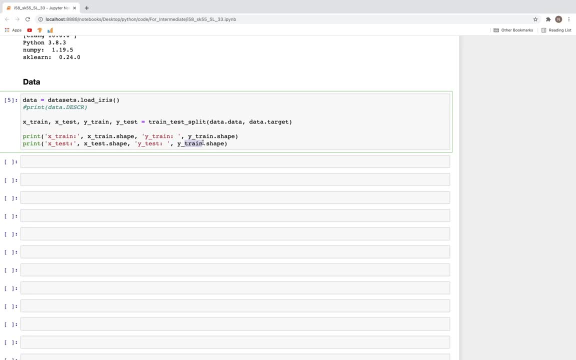 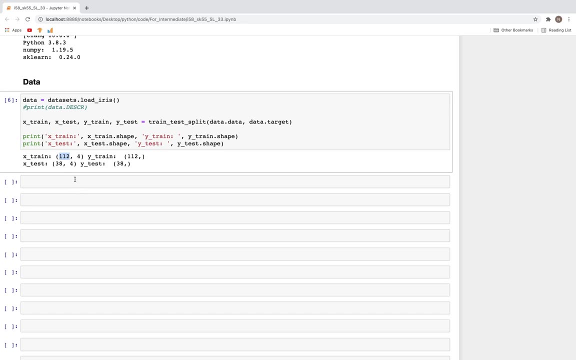 here and here. so we have four features and we have about 112 columns. sorry, i'm sorry, i'm sorry, i'm 111 rows now we are ready. two rows now. we are ready. two rows now we are ready to perform the lda: linear discriminant analysis and quadratic discriminant. 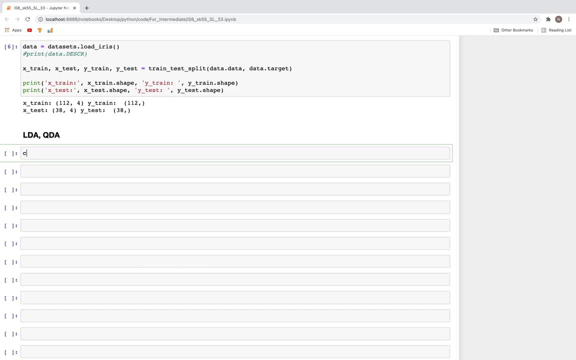 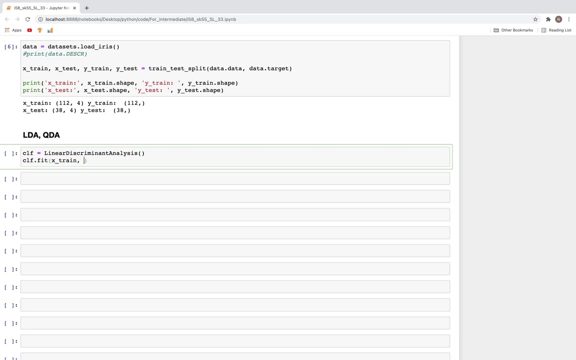 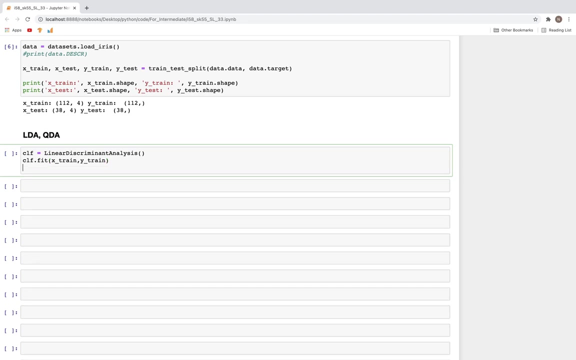 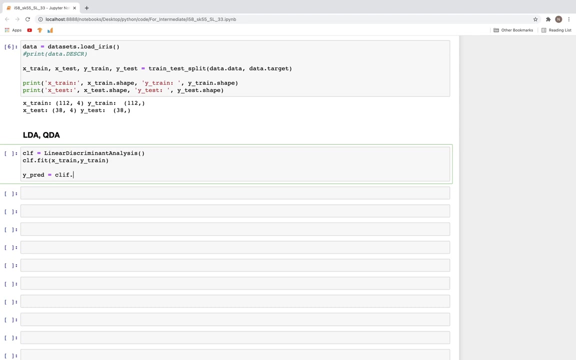 so for this we will create the variable. clf is equal to linear discriminant analysis. we'll use the default settings and clffit x underscore phone, x underscore train, y underscoreыв underscore train and then we can use that to predict. so y underscore predict pred is equal to clf dot. clf dot predict y underscore test. sorry, x underscore test. 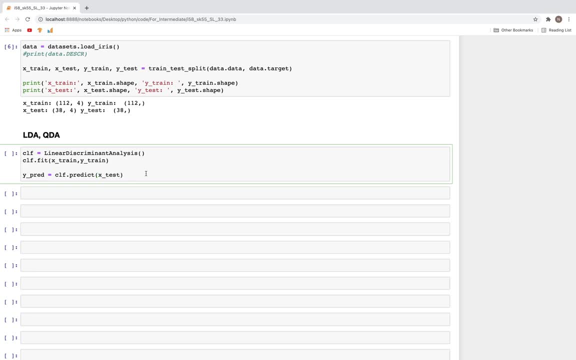 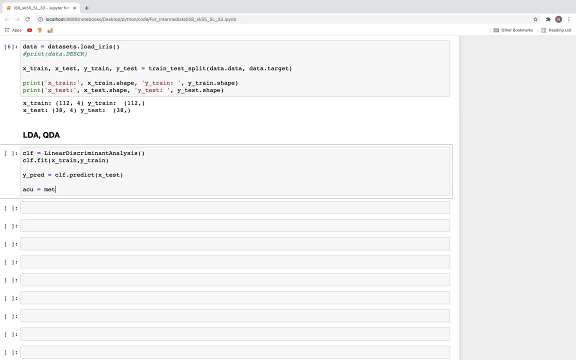 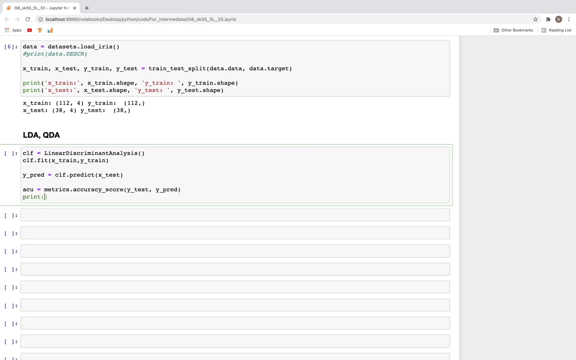 and once we have the predictions we can then go ahead and get the matrix. so let's look at the accuracy score. so matrix dot, accuracy, underscore score, and this would depend on the x y test and y pred. now we can print that out. so accuracy, and in addition we can also get 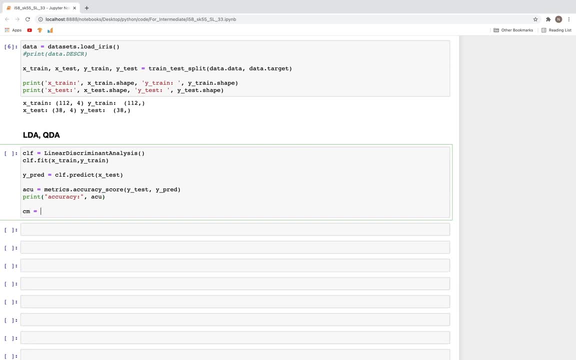 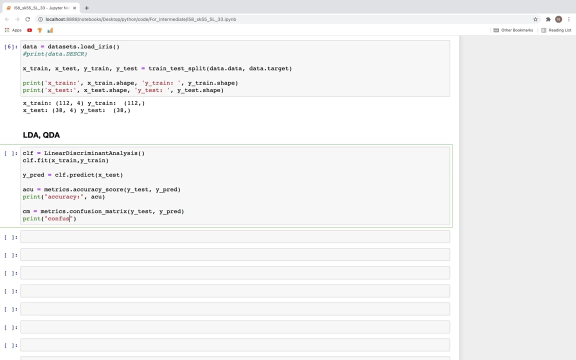 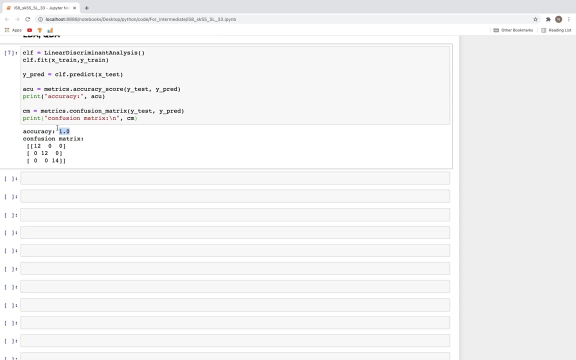 the confusion matrix. so matrix dot, confusion underscore score, matrix y underscore, test y underscore thread. and again we can print that. so this will be the confusion matrix and it's printed on a new row that is cm. so we get 100 accuracy- accuracy just because this is a small data set. if we apply this on a larger data set. 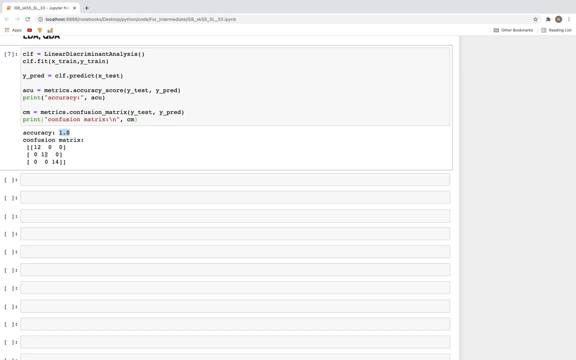 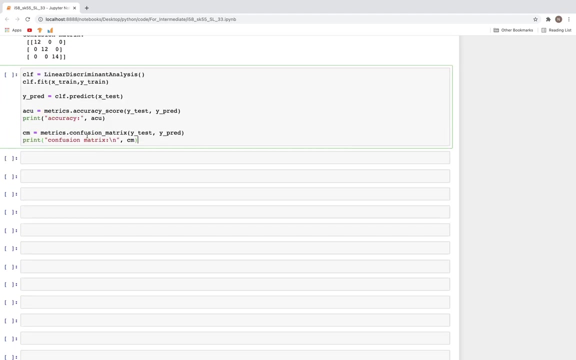 the value may not be one, and because here we can see in the confusion matrix that all the off diagonal elements are zero, which means that all the samples were classified correctly. now let's look at qda. so what i'll do is copy and keep everything the same, except change this to quadratic. 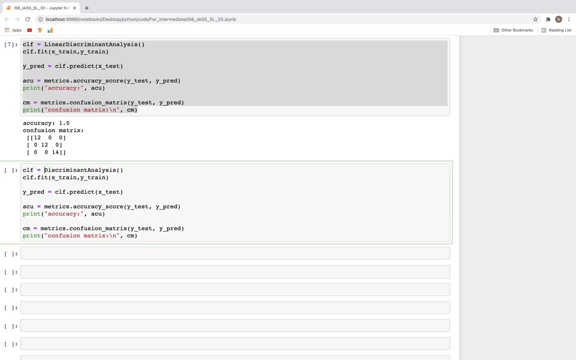 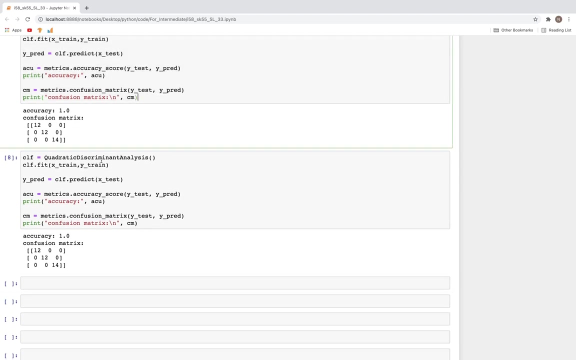 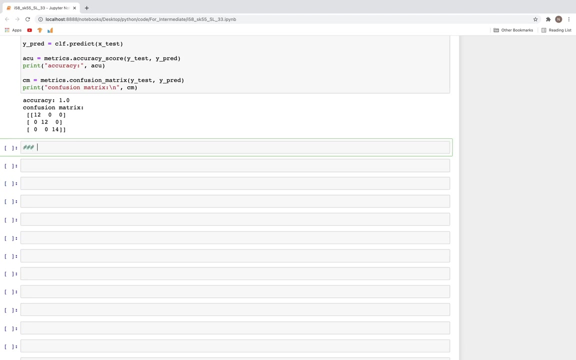 so quadratic discriminant analysis, and when we run this again, we get a hundred percent accuracy, which is kind of expected, because quadratic for such a small data set would uh, this, both, both of these could be overfitting as well. now, finally, let's look at dimensionality reduction. 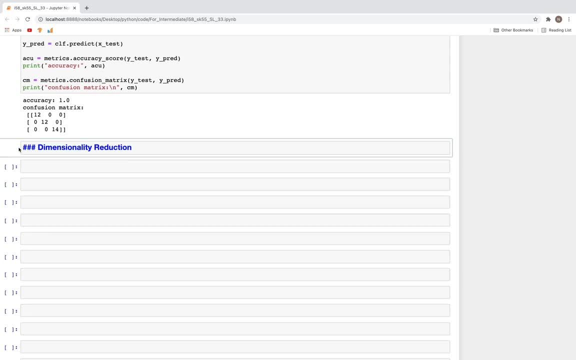 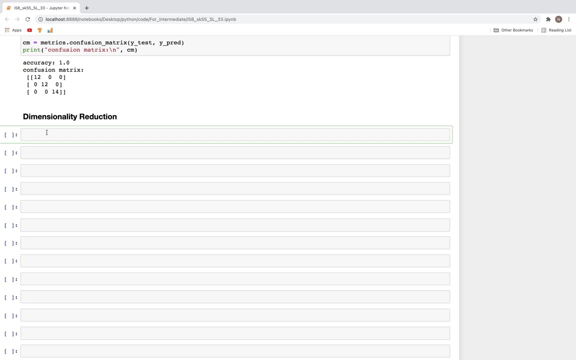 and for this we know that there are four columns of features, so four features, and we'll see what it gets reduced to to. so let's call this transform data trans c acfc as well. it gets here, assume this Reit. so we will call transform data trans c acfc. and, Hmm, change the time limit. two, two, three. orgnheen time limit Esto. this means that the реально returns, meaning that time limit 3 to 30 and Comparison mean regular time limit. 4 is one year is an annual pain period. so essentially the time limit 48 hours later from us, that's the fifth- is veryunku minus if we write 2, 3 a, not 15 days. 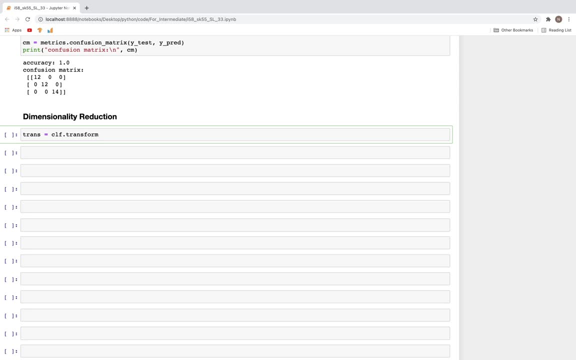 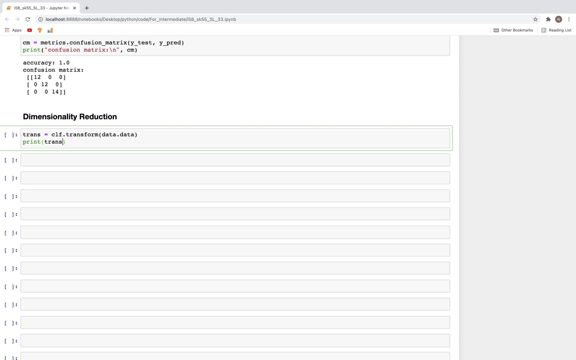 lf, dot transform. and what we need to transform is the very first data. so this was the data that we had: data, dot data. so what we can do is look at the shape after it is transformed. so transform dot shape. so let me go ahead and write the name: transformed data and here we can write the shape. 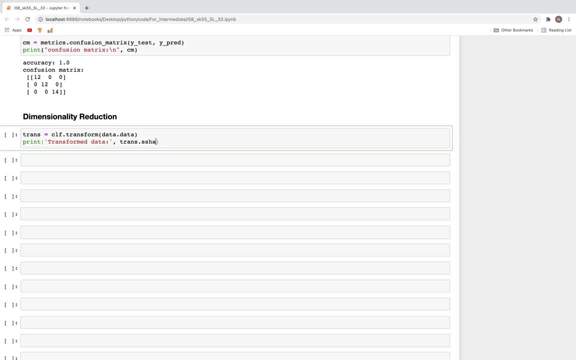 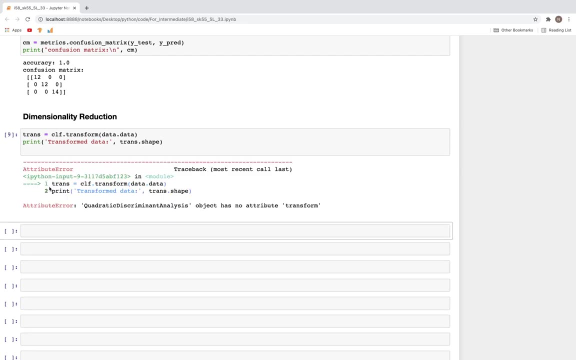 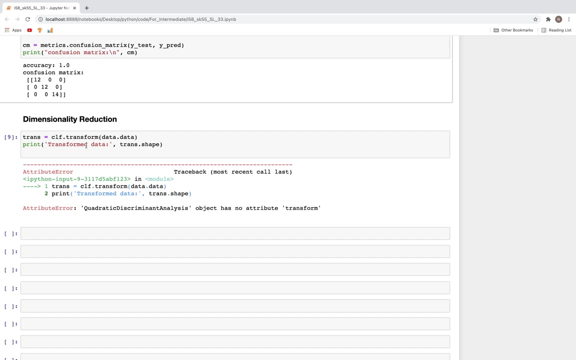 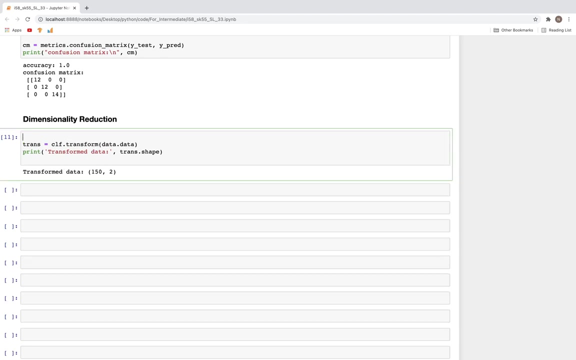 t-r-a-n-s dot shape, so that let me get the shape for the transformed data and we can run this. okay, because quadratic does not have this, and what i'll do is run the cell above. so now we have the tlf for linear discriminant analysis, and so let me type that here. this is: 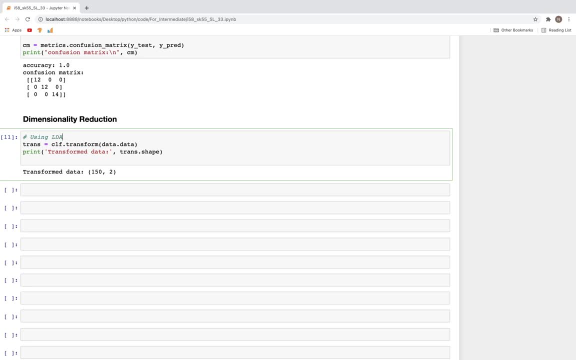 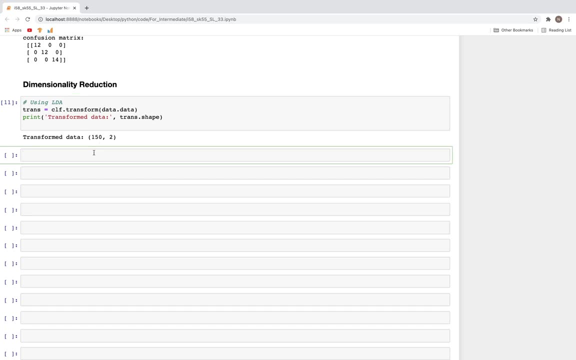 using linear linear discriminant analysis. so so we now have a transform data set with only two features. we started out with four features. we just have two. we could plot this, so let's uh plot it, uh, plt, dot, scatter, and here we have transformed pr, ans, and then all the rows in the column zero and then ns, and here we have all the rows and 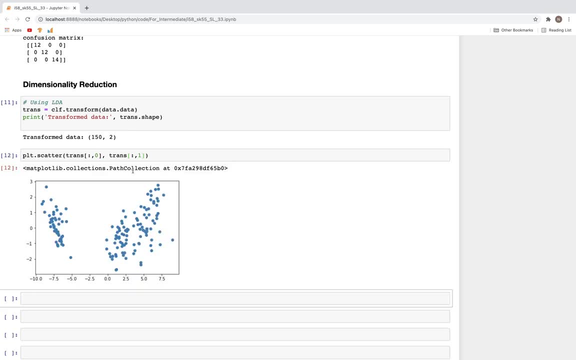 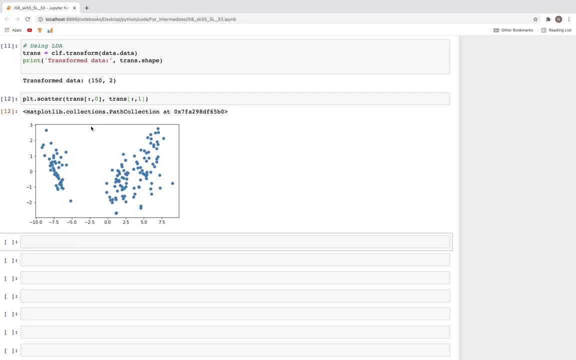 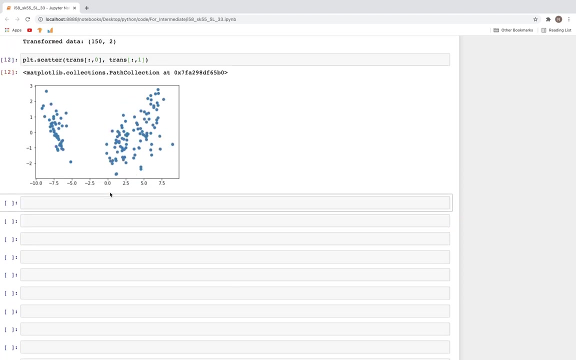 in column one. so when we run this, so as we can see there are two separate clear clusters and a straight line would be the best kind of decision boundary- we don't need any quadratic to separate these out. so let's go ahead and try to run the same linear discriminant analysis on. 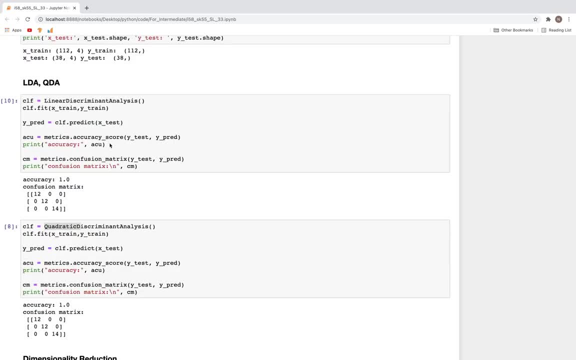 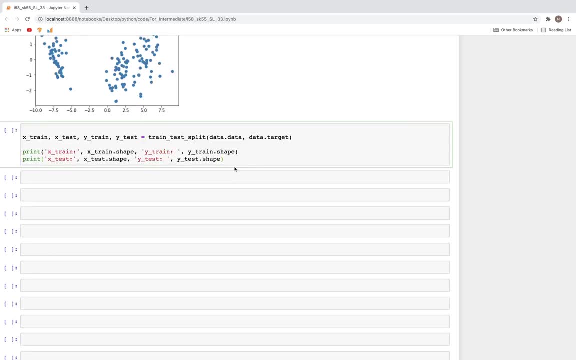 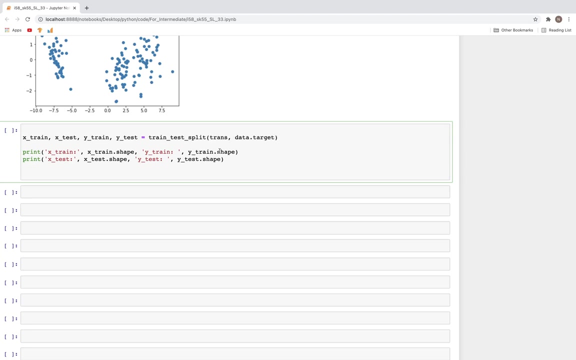 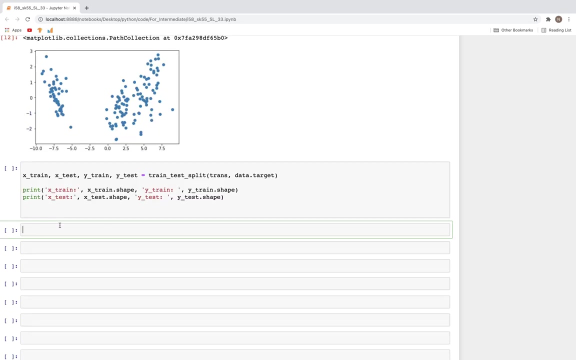 this transform data set and see how that goes. so for that we also need to get the train and test that again. so i'll write that here. the data in this case is going to be transformed data set, so i'll just use t r a n? s and then, for the actual fit, i'll copy this code from the above and paste. 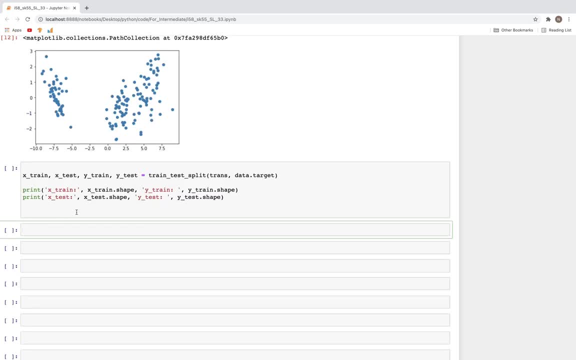 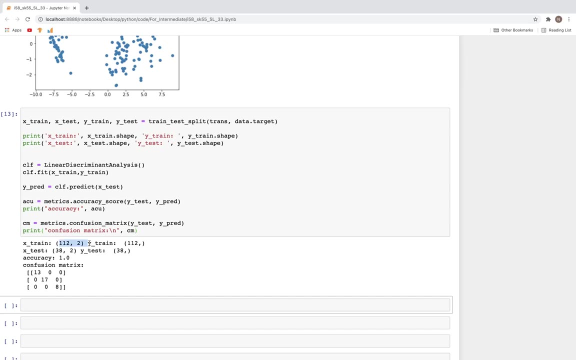 it here, so or maybe paste it in this cell itself. and when we run this: uh, as you can see, we have 112 rows, but the number of columns are reduced. we just have two columns, uh here, and the accuracy stays the same, uh, one. and this is the confusion matrix.